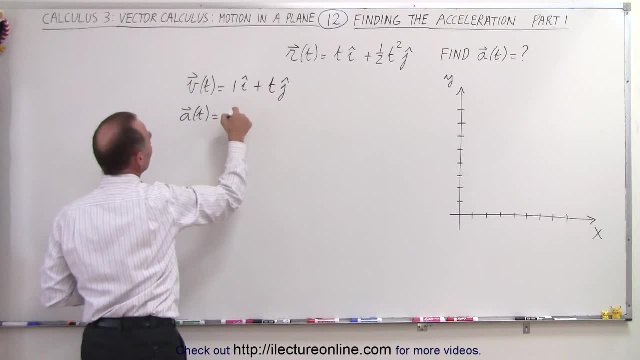 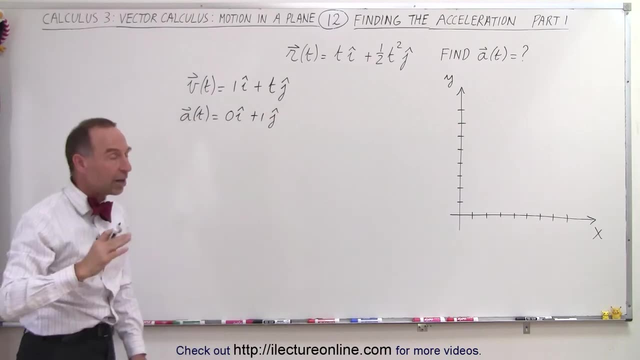 again, The acceleration vector as a function of time is equal to zero in the y direction and plus one in the j direction. So you can see that there's a constant acceleration in the y direction only and zero acceleration in the x direction. So what does that look like on the graph? on the xy graph, What we're going to do. 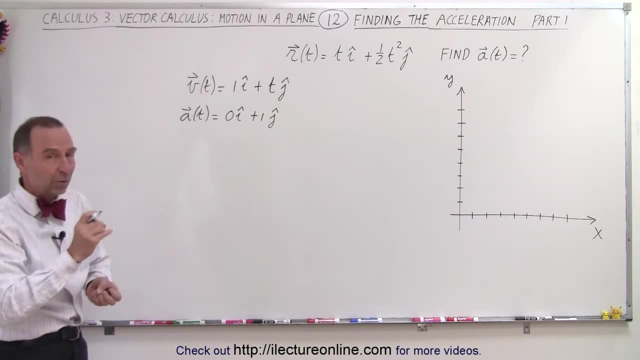 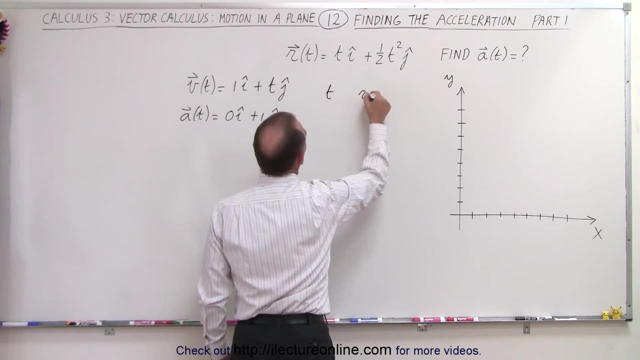 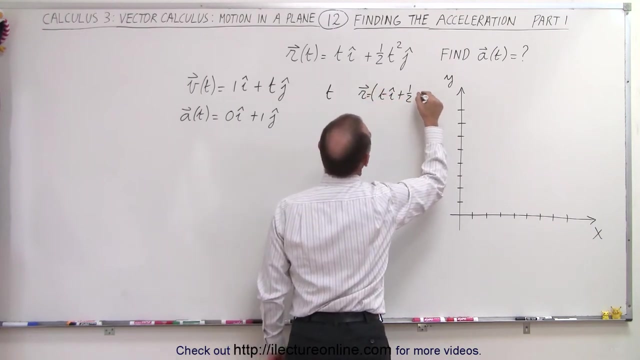 is, we'll set up a table of values, plug in some values for t and see what position the particle will have as it moves along the curve. So here we have the variable t and then r, which of course is t in the y direction, plus one half. whoop like this plus one half. 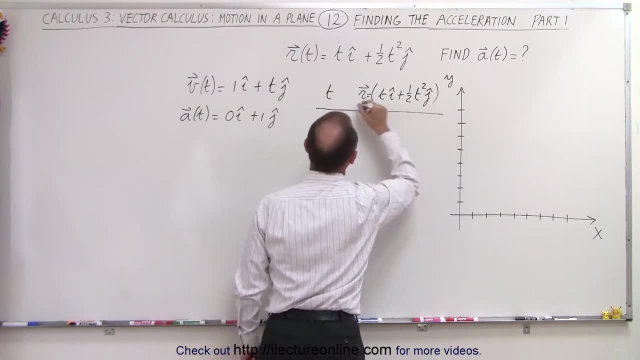 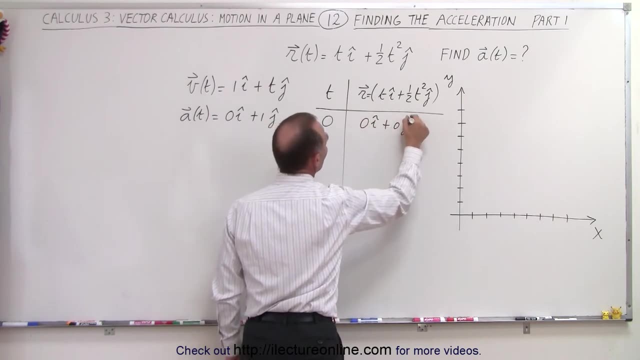 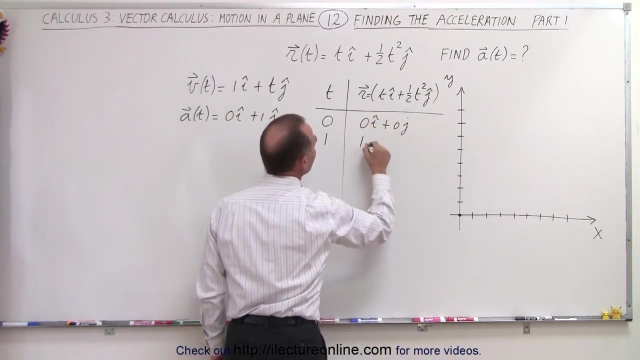 t square in the j direction. So when t is equal to zero, that gives us r is equal to zero in the i direction plus zero in the j direction, which means we are at the origin. When time is equal to one, that means that this will be one in the i direction plus one half in the j direction. 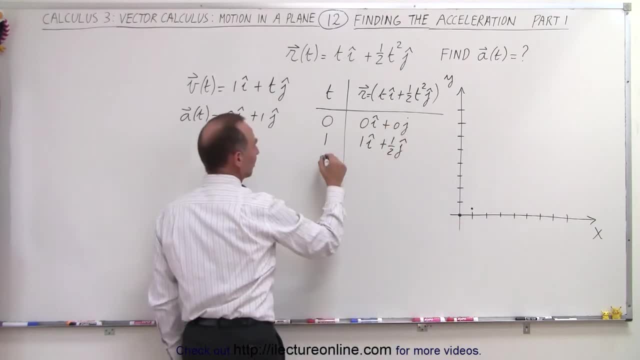 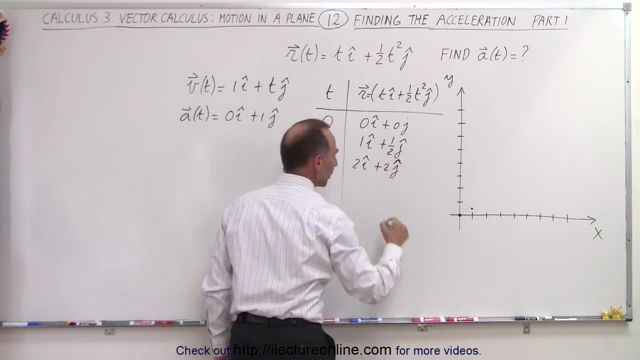 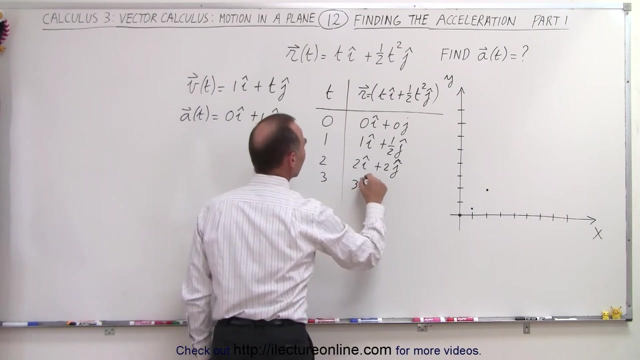 So that's one. that would be right there. If t is equal to two, that would be two in the i direction plus two in the j direction. Whoop, there we go. So it would be two and two. that would be right about there. If t is equal to three, that'll give us three in the i direction plus 4.5 in the j. 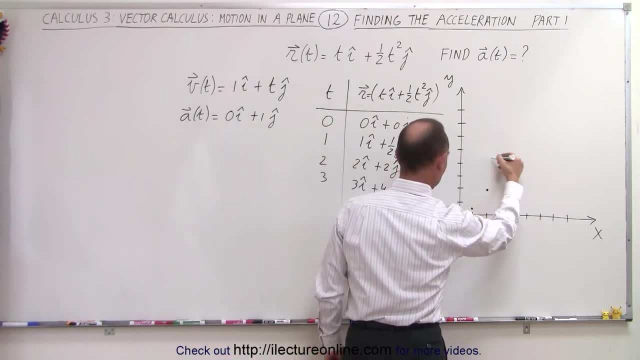 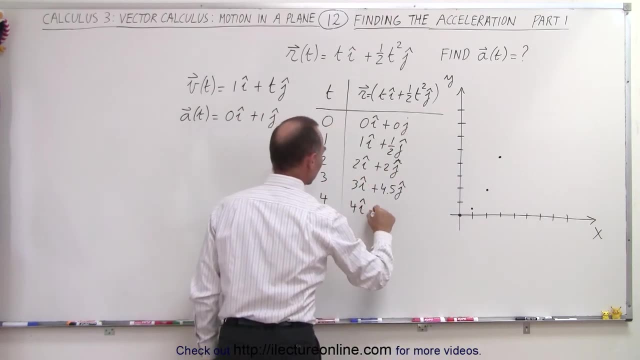 direction. So that would be three and 4.5. that would be about here. And then we have when t is equal to four. that would be four in the i direction plus eight in the j direction. So it would be four and eight. 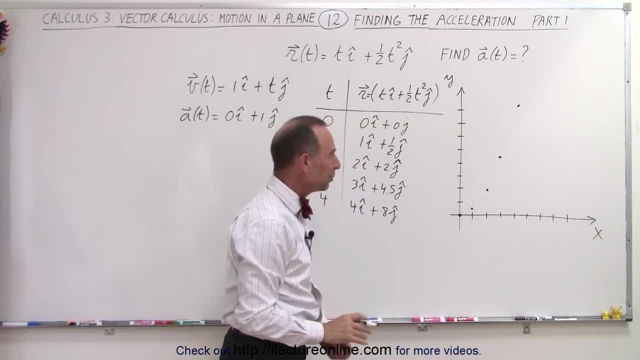 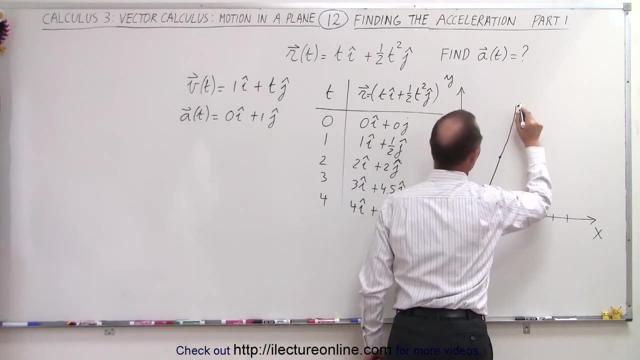 Right there. Notice, by the lines that I drew I knew it was coming, But you can see now the curve. that's the s curve, if you want to call it that. That's the path of the particle Whoop. let me just 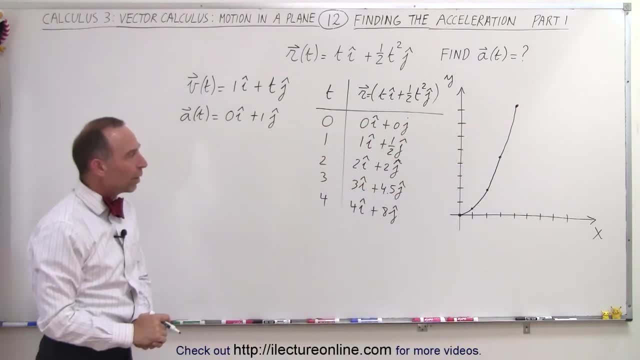 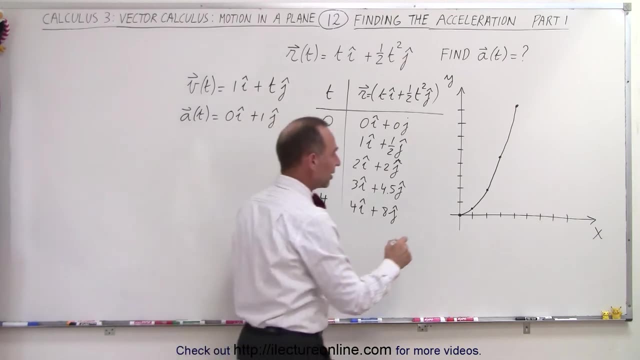 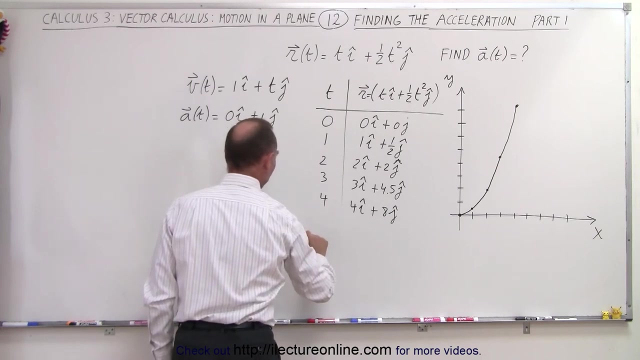 move the point over a little bit. There we go. And now, what does the- hmm, let's say, velocity vector look like? What does the acceleration vector look like along some of these points? Let's take this point right here. Notice our velocity vector of v when time is equal to zero. So if t is equal to 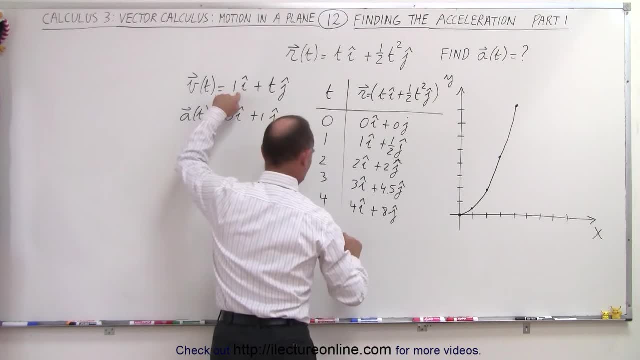 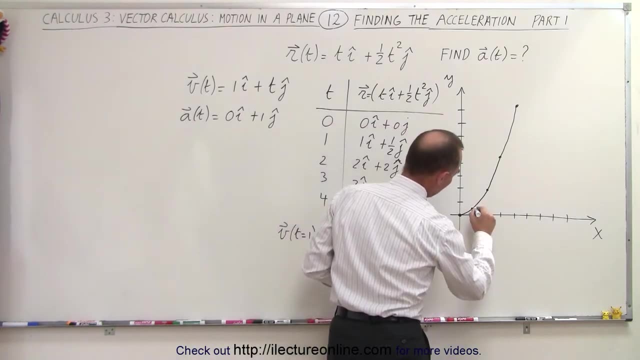 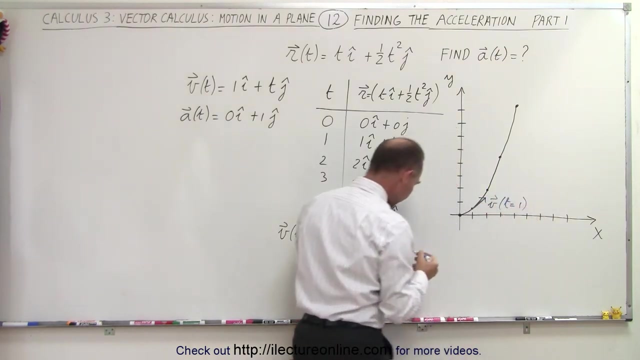 one. it's going to be equal to one in the i direction plus one in the j direction. So my velocity vector- and let's use a different color- will look something like this. So this will be my velocity vector when time is equal to one. What will my acceleration vector look like at that? 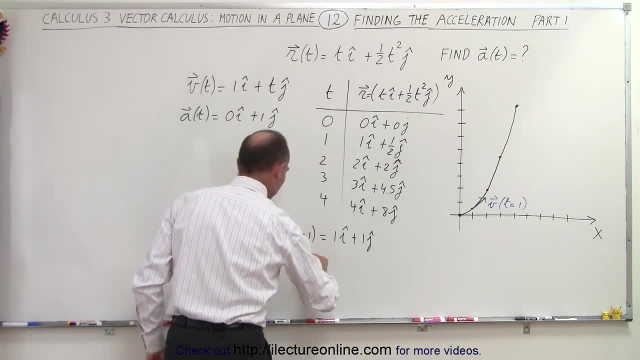 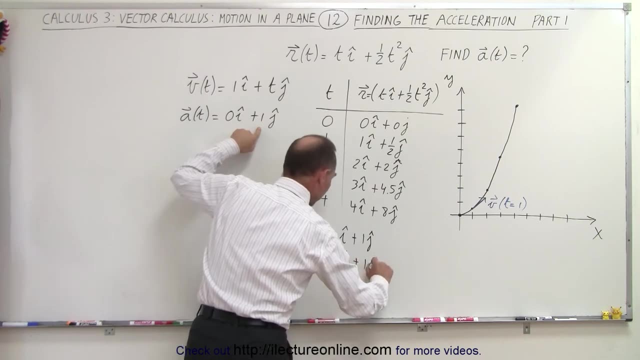 time. Well, my acceleration vector, when time is equal to one, is equal to that would be zero plus one, So zero in the i direction. So that would be zero plus one, So zero in the i direction. So that would be zero in the i direction plus one in the j direction. Notice, the acceleration vector doesn't. 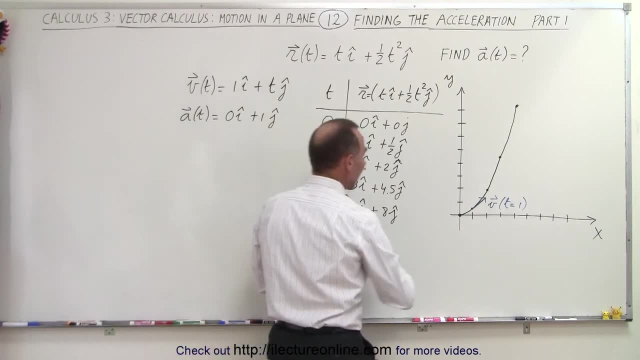 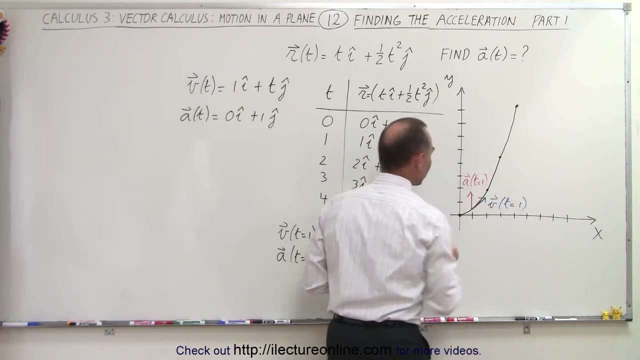 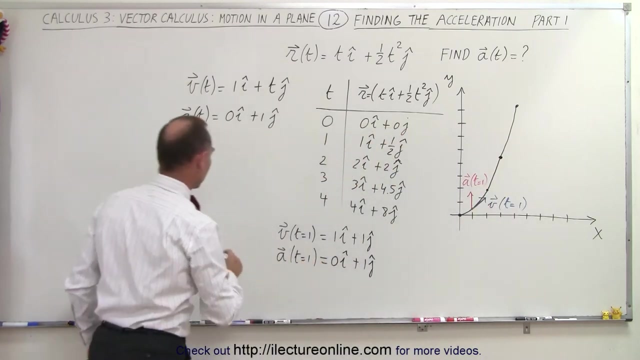 change with time. It's not dependent on time, So it's always going to have a vector that looks like this. So this here will be the acceleration vector when time is equal to one. So let's now move to a different point. Let's move to the third point right here, where t is equal to three, And again. 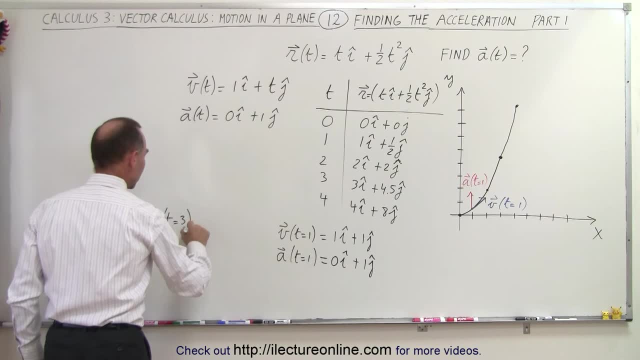 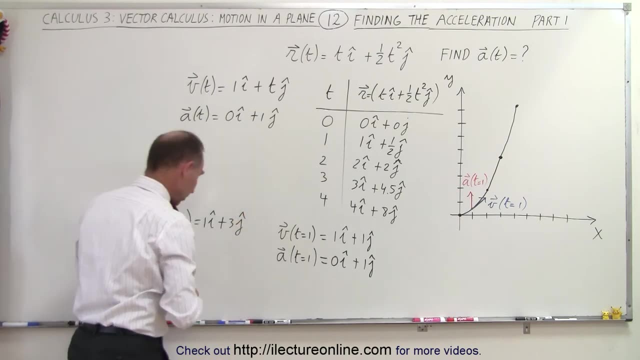 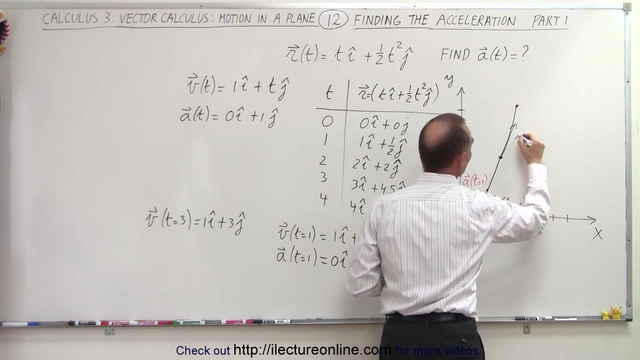 we'll take the velocity vector when time is equal to. three is equal to, that would be one in the i plus three in the j direction. So you can see that at that point my velocity vector will look something like this: It will move faster in a much more steep direction. So velocity vector when time 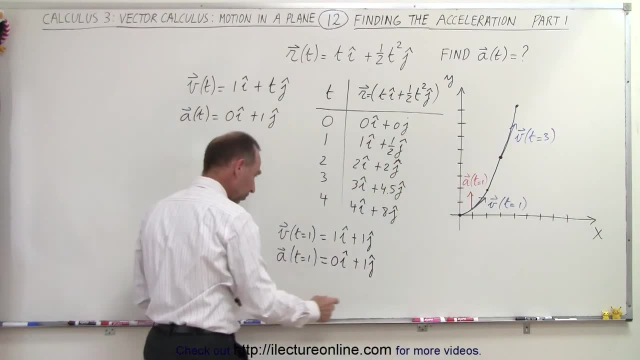 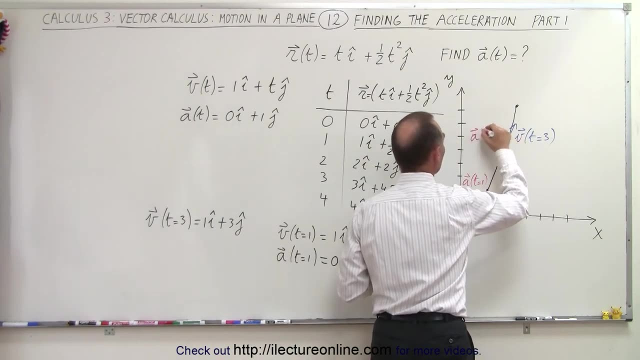 is equal to three. And then we realize the acceleration vector will still be a constant. Where did my pen go? So my velocity vector will still be like this. Those will be a when time is equal to three. In other words, there's no change in the acceleration vector, And that's kind of a 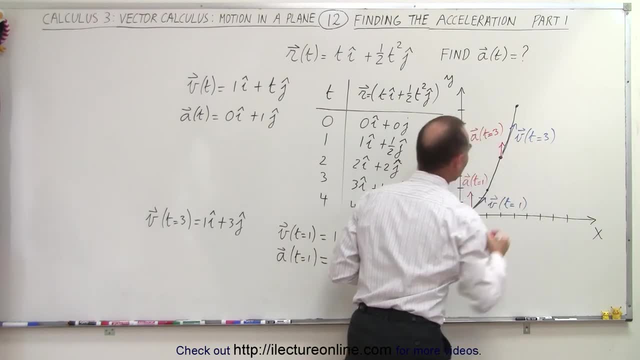 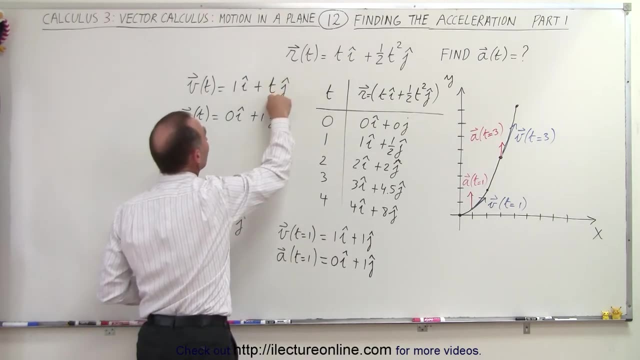 little bit crooked. Let me try that again There A little better. So notice: my velocity vector is constantly changing because the y component depends on t, The x component will always be one And my acceleration vector will be one in the y. 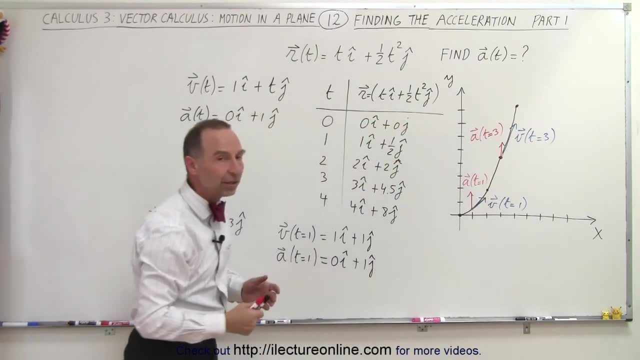 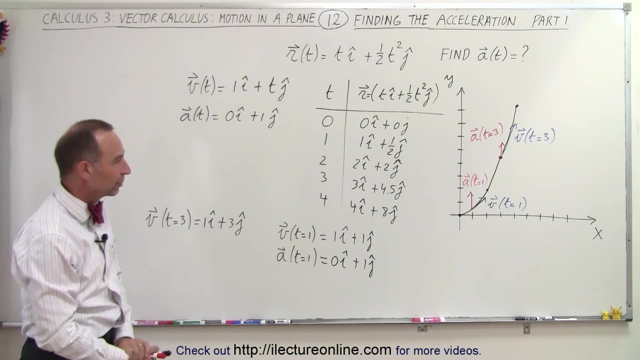 direction, no matter where we are on the curve. So that gives you a feel of how to look at the motion along the curve and how to find the curve defined by the parametric variable t. Anyway, that's how we find the acceleration vector. when we're only dealing with time,